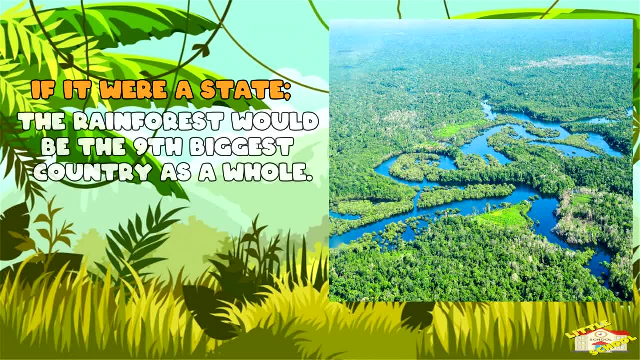 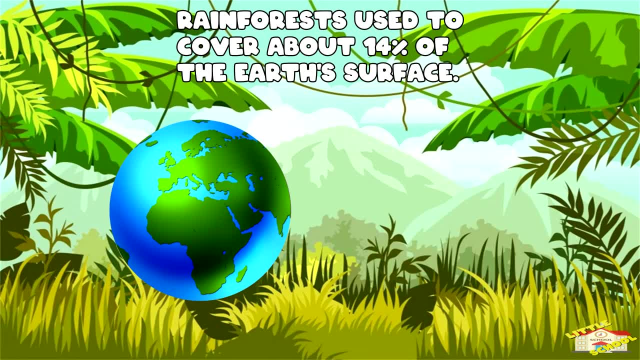 ground. The Amazon rainforest is so huge that if it were a state, it would have been the 9th biggest country. Rainforest used to cover about 14% of the earth's surface, but now they are disappearing Due to heavy tree cutting. they only cover. 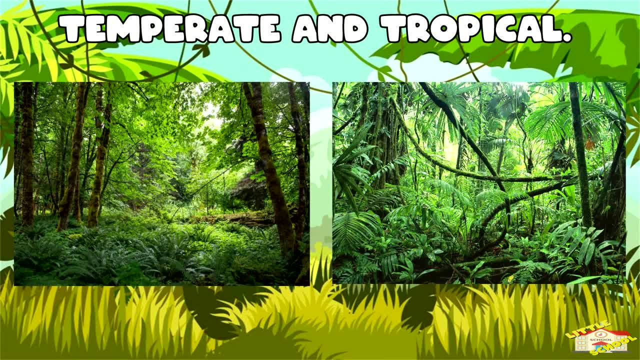 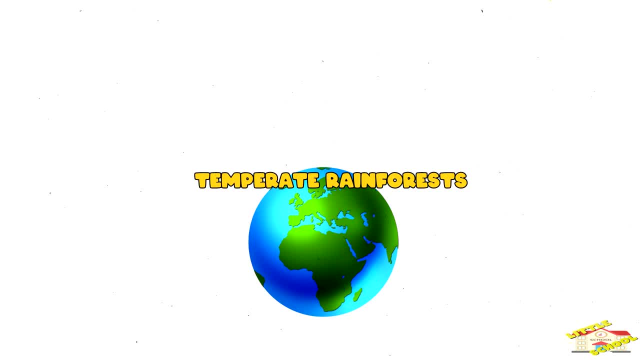 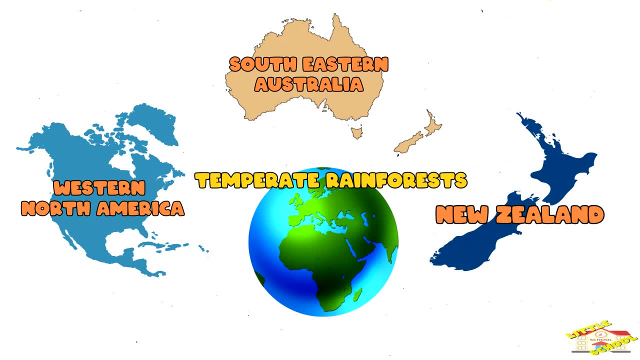 around 6%. There are two types of rainforest: temperate and tropical. Temperate rainforests are found in a couple of regions around the world, such as Western North America, Southeastern Australia and New Zealand. The types of animals that you can find in 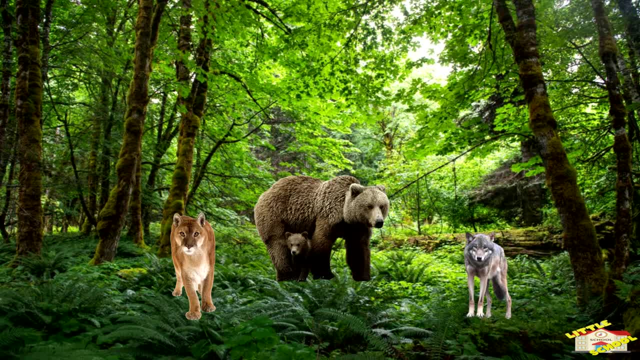 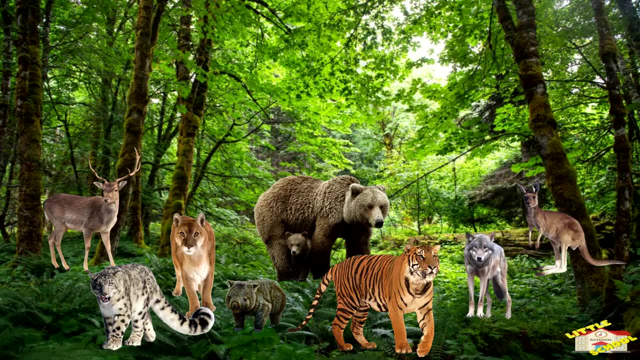 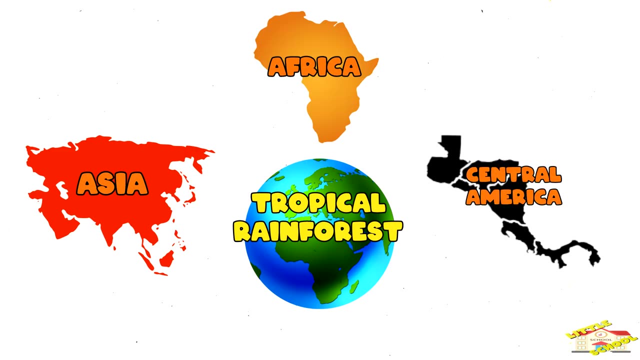 temperate rainforests are pumas, bears, grey wolves, elk, Siberian tigers, snow leopards, kangaroos and wombats. Tropical rainforests are found in areas close to the equator, like Asia, Africa and Central America. 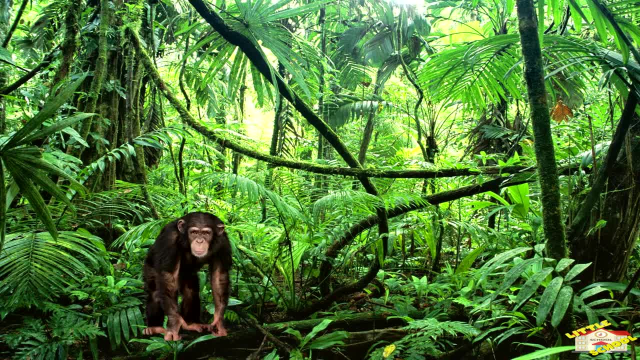 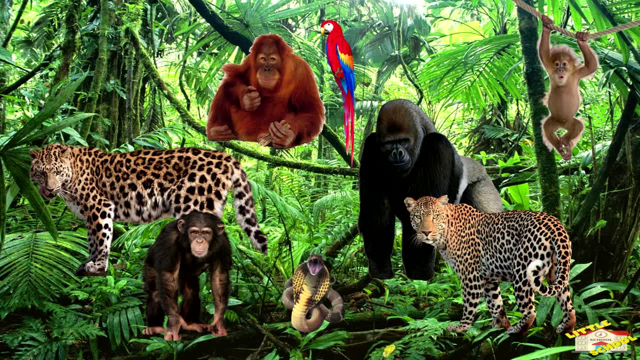 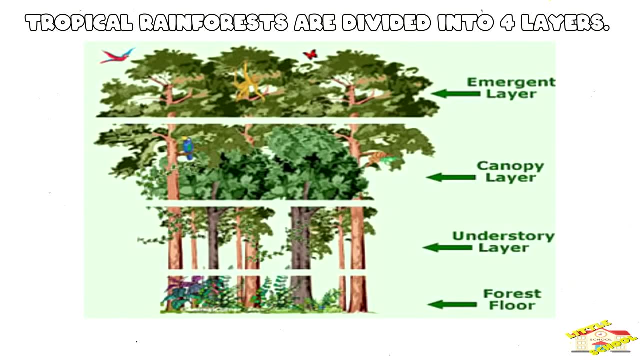 The types of animals that you can find in tropical rainforests are chimpanzees, gorilla, Indian cobra, orangutan, jaguar, monkey, leopard, parrot, iguana and the tree frog. Tropical rainforests are divided into four. 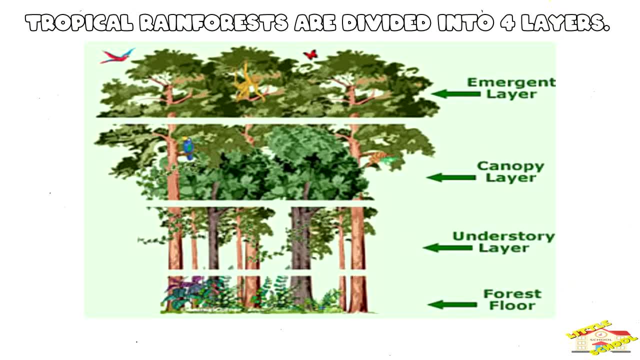 layers called the emergent, canopy, understory and the forest floor. The emergent layer has lots of tall trees that grow above the canopy. The canopy zone of the rainforest contains the upper parts of the trees. The understory layer in the rainforest is under the leaves of the trees but above the. 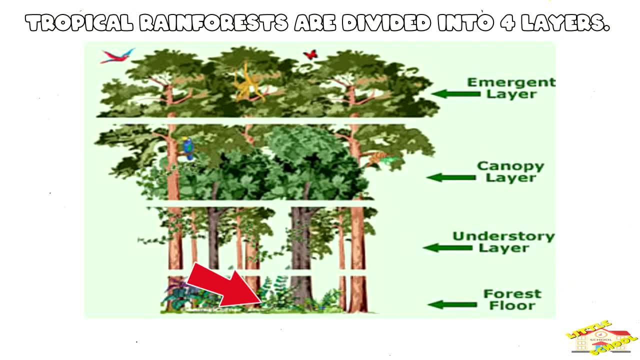 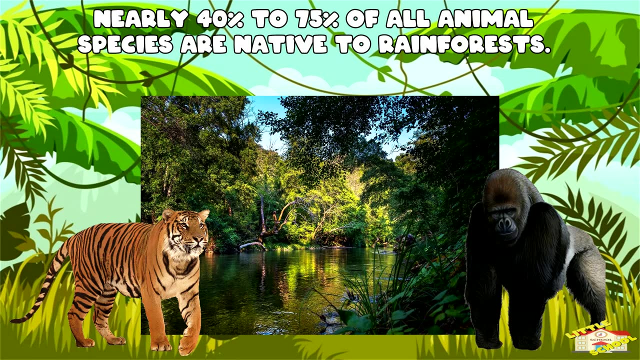 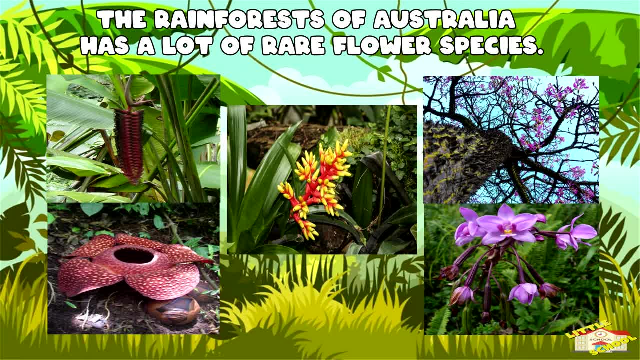 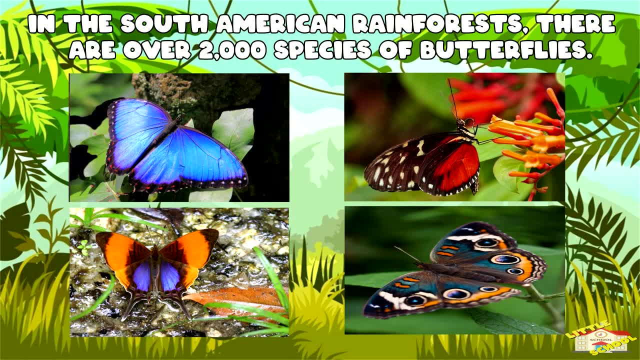 The rainforest of Australia has a lot of rainforests. The rainforest of Australia has a lot of rainforests. The rainforest of Australia has a lot of rainforests. The rainforests of Australia will never be covered, Since they are almost completely.